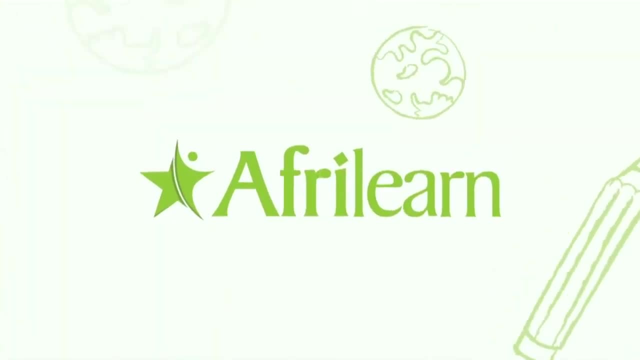 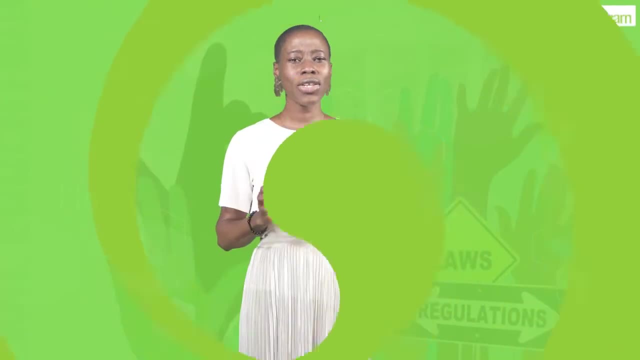 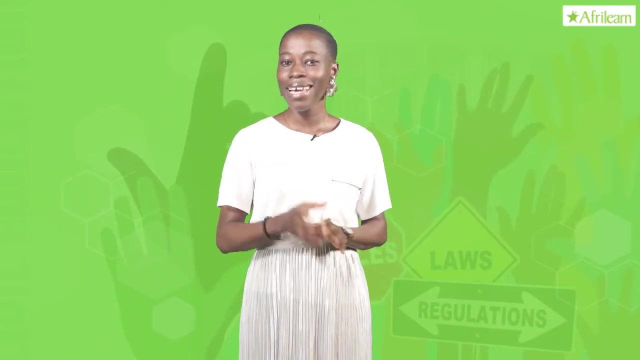 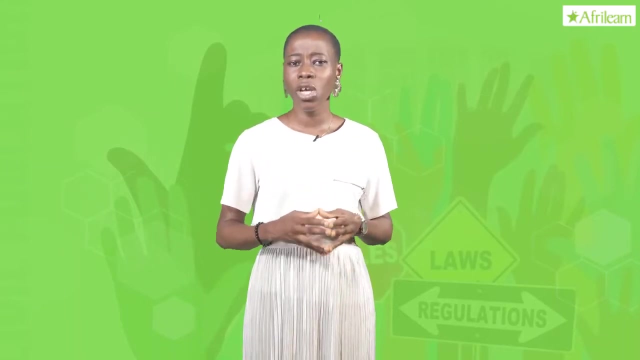 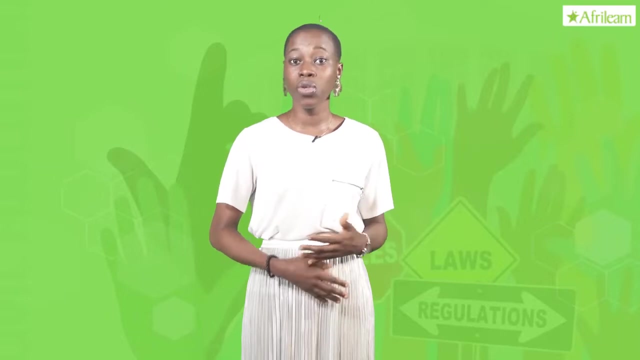 There are a lot of skills one could learn to make one independent. Do you still remember Go-Pep The graphic designer? So Go-Pep learned artistic skills, which helped to instinct in him the ability to process creative qualities that enable him to excel in producing creative. 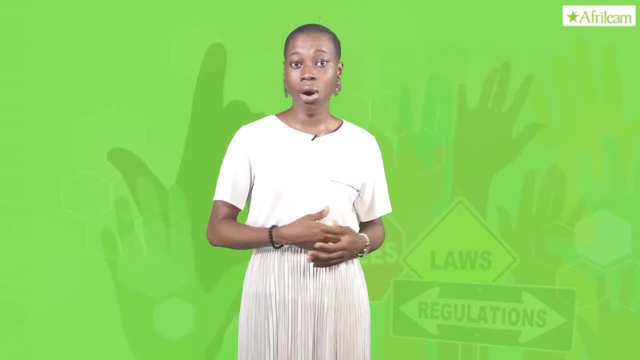 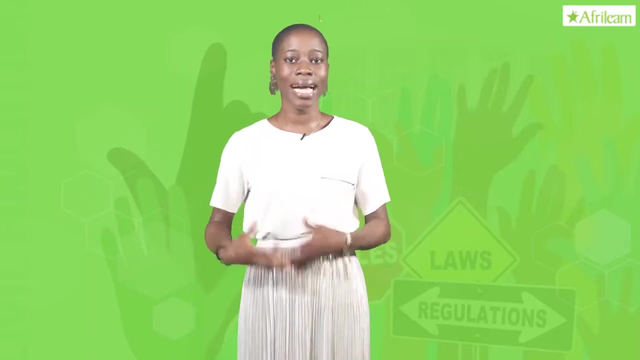 works. Some other skills could be vocational or entrepreneurial skills, Skills like makeup artistry, hair designing, catering- that teach one how to be independent by making one skilled business owner or producer of other kinds of goods or services- Go-Pep, for instance. 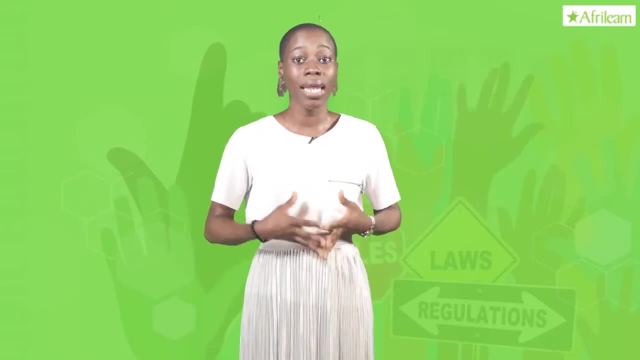 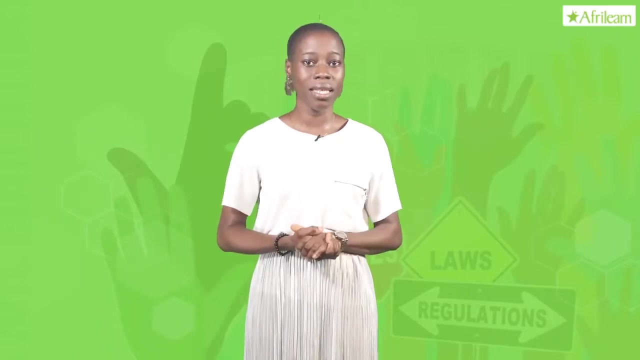 also learned some life coping skills as he went about learning his graphic designs. It helped him to deal with realities, expectations and challenges of life. Even as a student, he was able to cope with his books, house chores and learning graphic designs From. 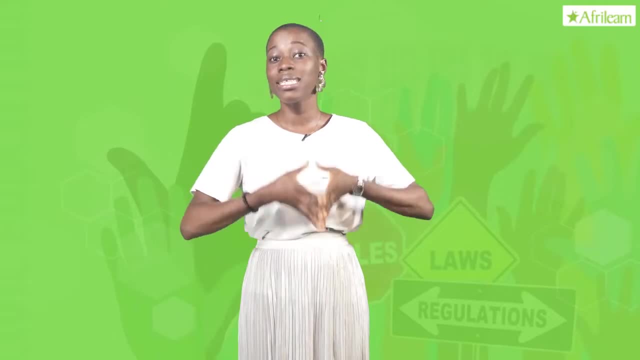 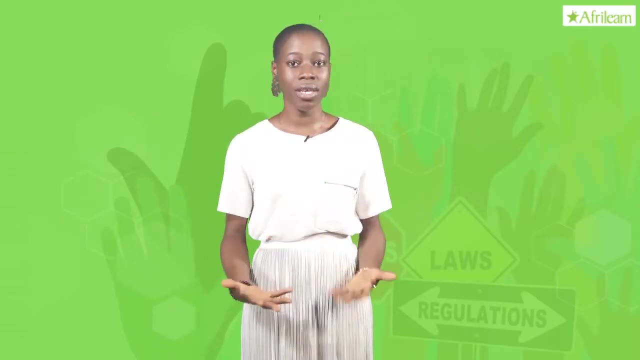 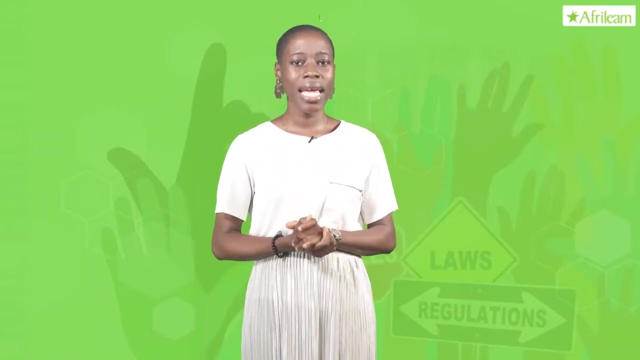 school also, he was able to learn and build his intellectual skill. The knowledge he got from school helped him to acquire the ability to think and to understand ideas, perspective and process information. Go-Pep had a friend. her name was Ella, Although Ella did not. 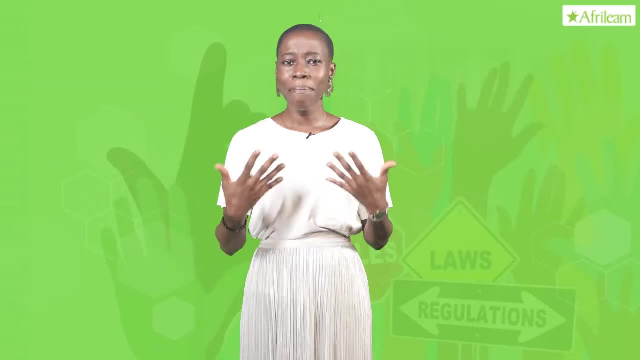 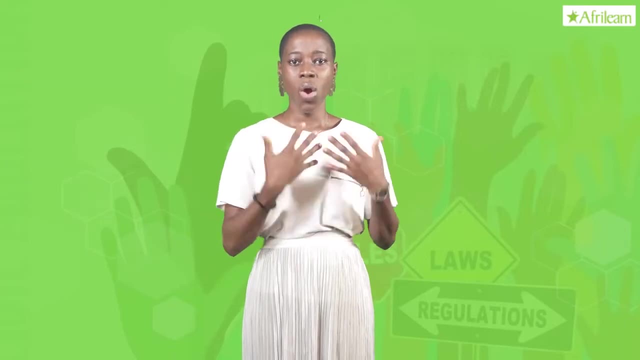 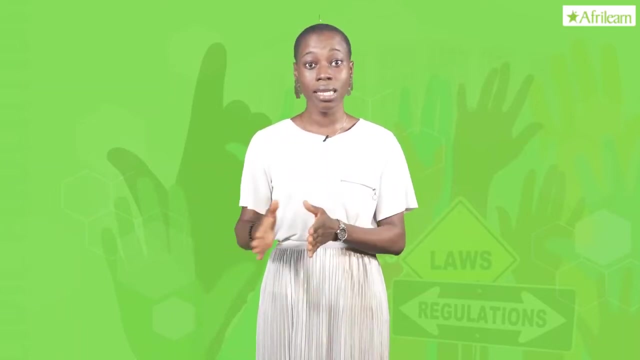 learn graphic design like Go-Pep. she had an amazing leadership skill. She was the captain of a class and knew how to manage people and relate with all her classmates. She was also very skilled in goal setting and decision making. Outside this, Ella was a good communicator. 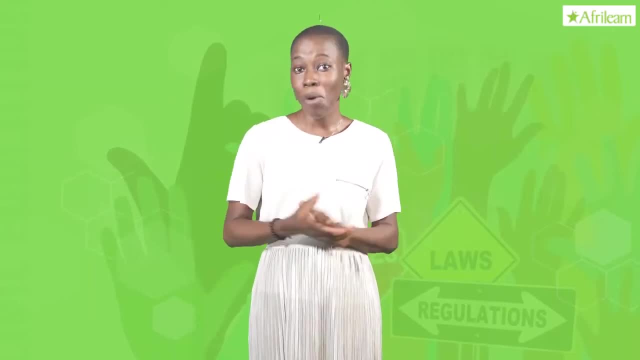 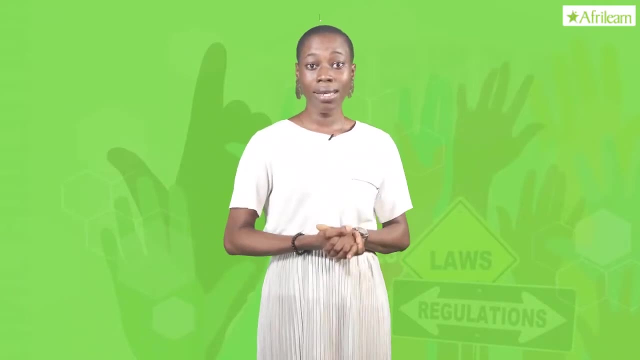 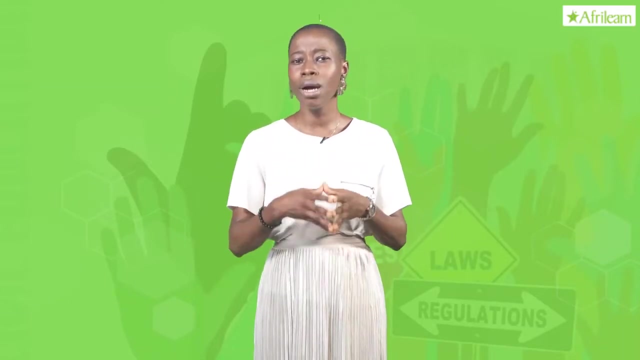 She could communicate very clearly, Not because of the way she spoke English, but because of the way she presented every situation. She knew how to convey messages effectively – when to talk, how to talk and who to talk to at the right time. Go-Pep, on the other hand, had amazing negotiation. 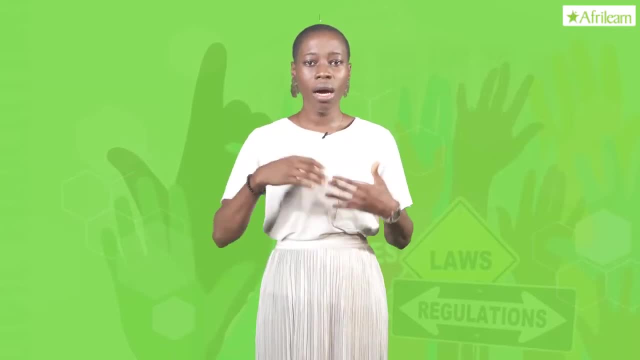 skills. For instance, when the owner of the office where he learned his graphic design skills wanted him to start a business, She was able to communicate very clearly and finally understood what she was trying to say. When she signed her contract, she was able to.